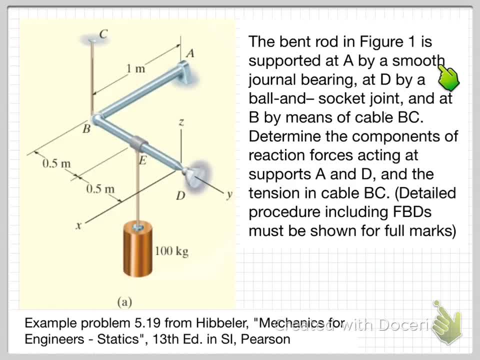 So the next thing that we look at in our information here is that we're told that we have the bent rod is supported at A. Supported at A. Supported at B. Supported at C. Supported at D. Supported at E. Supported at D. 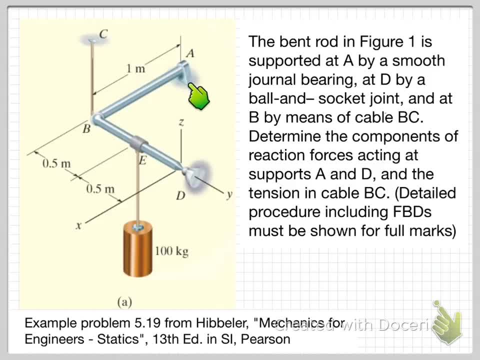 Supported at E. So that will give us some information about the forces and all moments that occur at this point. Secondly, we're told that at point D we have a ball and socket joint. So down here we're told that we have a ball and socket joint. so again, that will give us some information. 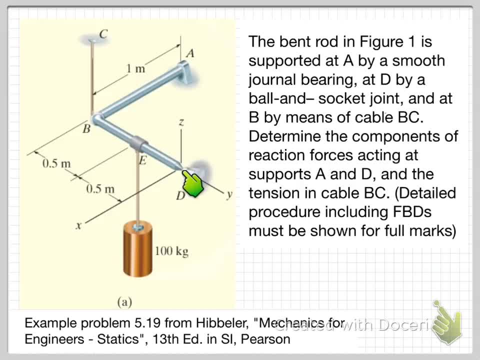 about the forces and all moments occurring at that connection. We're also told that it's supported at B by means of a C1. means of a cable BC. so we have our cable here supporting that part of the rod and in this problem we're asked to determine the components of the reaction forces. 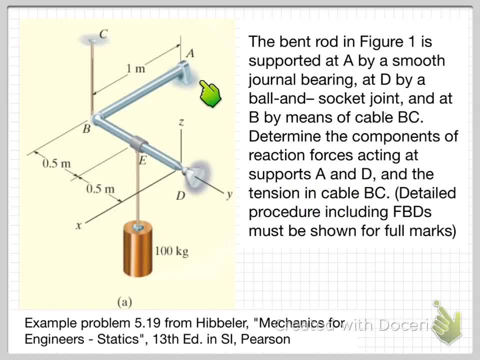 acting at the supports A and D. so our supports A and D that we identified before and the tension in the cable BC. okay, and as part of the question we're told that we're needing to include detailed procedure and free body diagrams to get full marks. so if this was a quiz question, but of course you. 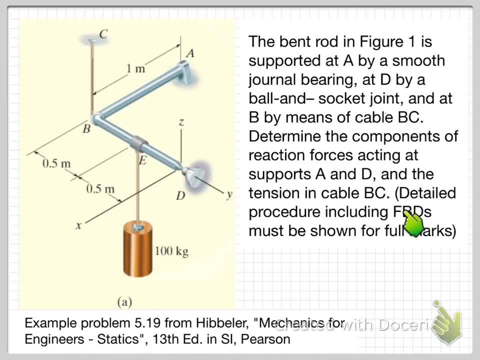 should be doing that anyway. in any of your engineering mechanics problems, good procedure and free body diagrams are essential. as with any engineering mechanics problem, there are usually many different ways to solve the problem. as you will note down here, this exam is actually taken from here below: mechanics for engineers: the statics. 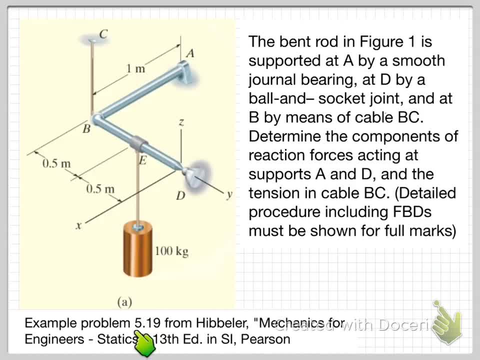 volume. if you look into in that textbook, you'll see that this problem is solved in that example using a vector approach. in this video I'm going to use a very simple, straightforward scalar approach which you can follow and you just apply your Newtonian mechanics and follow a simple step-by-step procedure and take 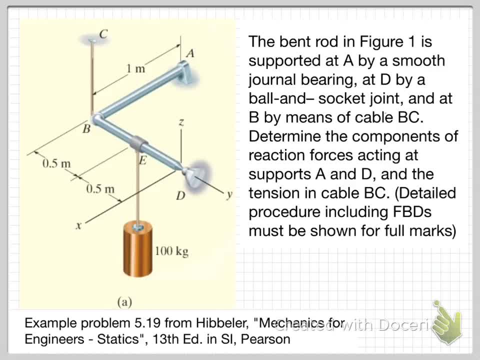 care to understand the where the forces and moments are applied and making sure that you obey Newton's laws. then you should be able to make your way to the solution and the correct answers without needing any particular insight or fancy methods to get to the answer. okay, so let's start by drawing our free body. 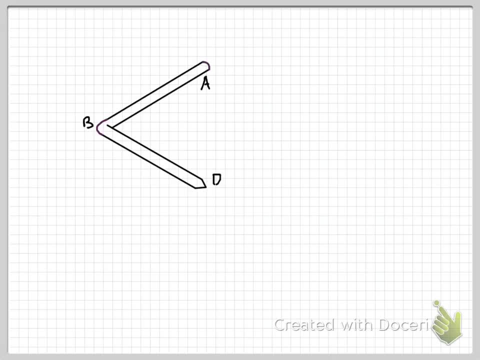 diagram once we have the basic shape, and you should use drawing instruments to do your free body diagrams. so once we have our basic shape and some important points labeled, we can then start to add in our forces and or moments. so when adding the forces and moments to the free body diagram, I usually start with the known 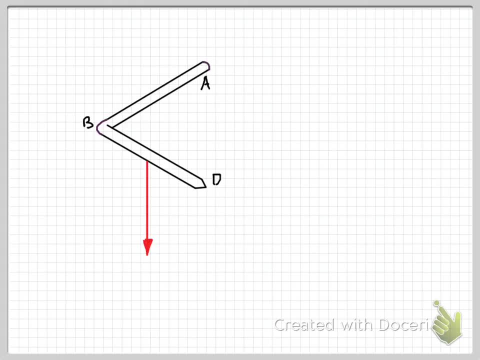 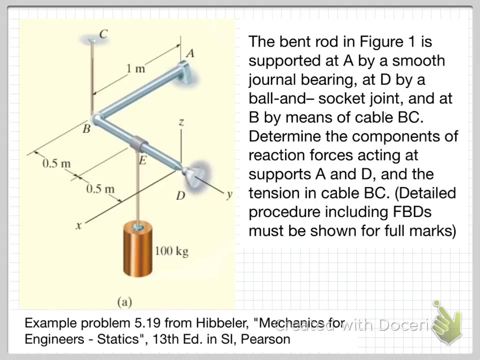 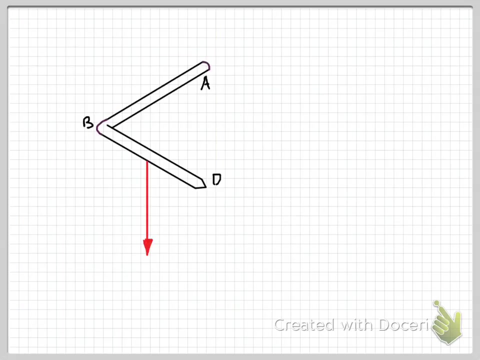 loads and then work from there. so we have our weight load hanging down and we can indicate what the value of that is. so let's just go back and check our information. so we are told that we've got 100 kilo mass and our free body. 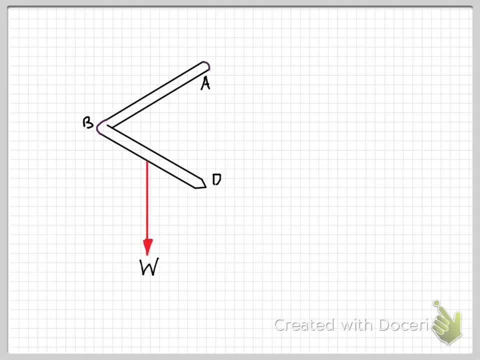 diagram has our force shown there as a W, and we can calculate that because we know that the force due to gravity will be mass times gravity, which is 9.81. so we can fill that in hundred times nine point eight one and of course we get 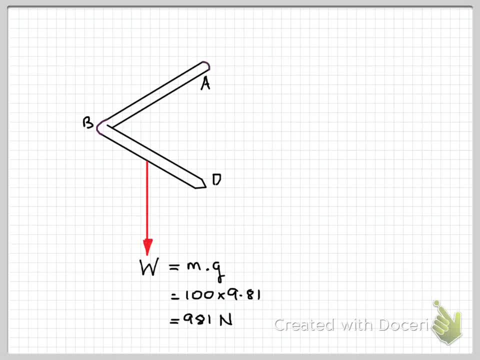 981 Newtons. So now we need to start adding in our unknown forces and moments. So we'll start with our cable at B, We know that the cable is a two force member in equilibrium, so the force will be acting along the direction of the 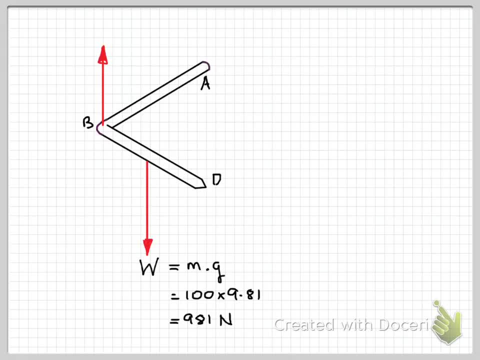 cable BC. So we can draw that in in our free body diagram. and of course we need to give our unknowns a name or a variable name. so we'll call that T subscript BC. Okay, so now we need to consider our reactions at our supports. 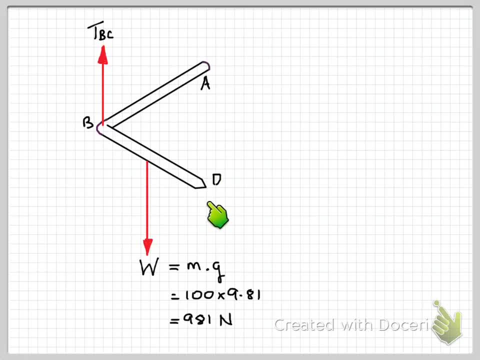 D and A. So let's start with the ball and socket joint at D. Now, if you're not sure what forces and or moments are supported by that type of constraint, you can go to the table in your textbook. So in your textbook you'll have a table that looks: 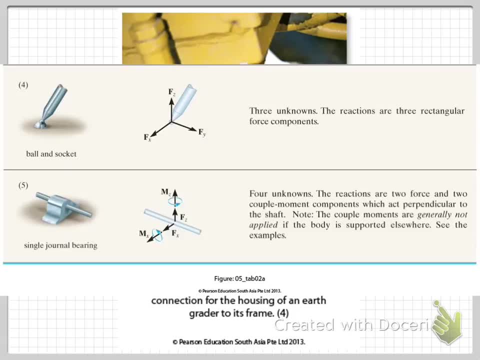 something like this, And you'll be able to see that for a ball and socket joint we've got three forces in each of the three component directions and no moment Okay, so it's free to rotate about that point If you're not sure what that looks like in. 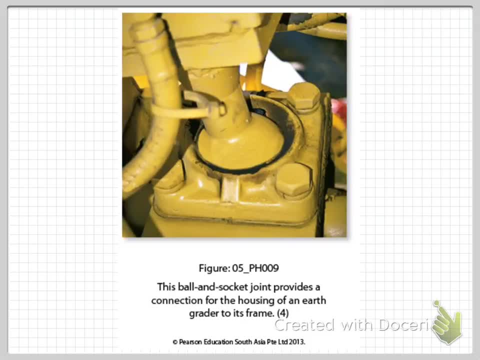 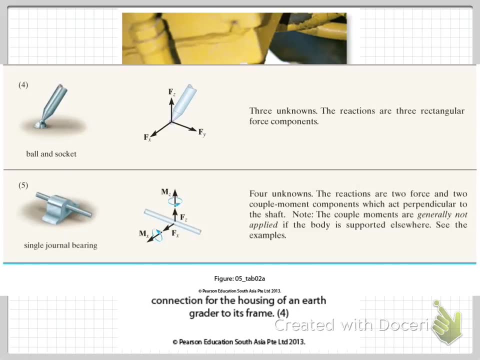 practice at the physical ball and socket joint. here's an example of that. Okay, but for the purposes of drawing your free body diagram, for your mechanics problem, your idealized representation. So here's your idealization and here is what we draw in our free body diagram to represent that connection. So back at our 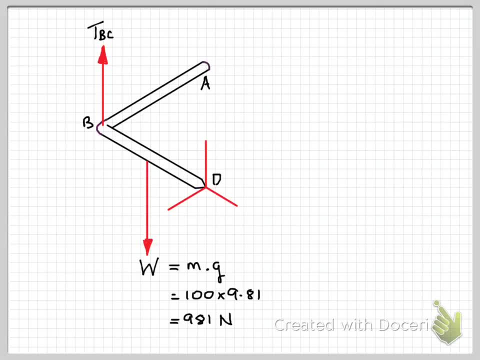 free body diagram. in our problem we can now draw in our forces in the three X, Y, Z directions and we can indicate those directions on our free body diagram. So we can see that we've got a free body diagram for reference. and once we've done, 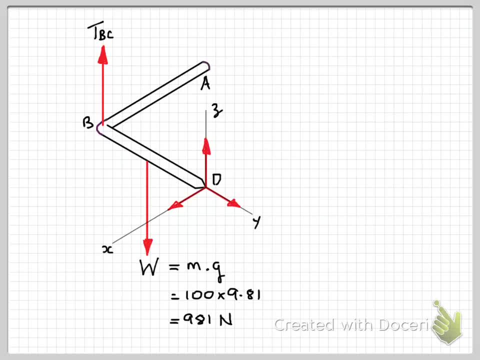 that we can also put on our arrowheads for our forces. So at this stage we'll just assume the sense of the force and then, once we've done that, we should of course then label all of our unknowns. So for the reaction force in the X direction, I've called that. 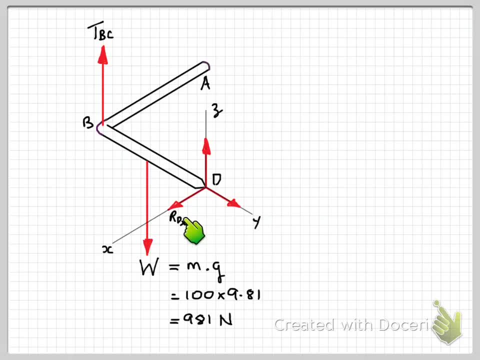 R, subscript DX. In a lot of textbooks and other examples you'll see people write just capital D, subscript X. You can do that if you like, but I tend to prefer to use capital R or capital F for the force, and then D or whatever other point it is that we're talking about and then the direction. 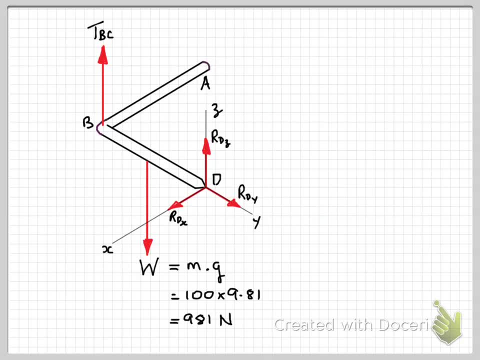 So do the same thing for the other two forces. and now we need to consider our support at A, and we're told that that was a smooth journal bearing. So again, if you don't know what the reactions should be for that, you can look at the table again. 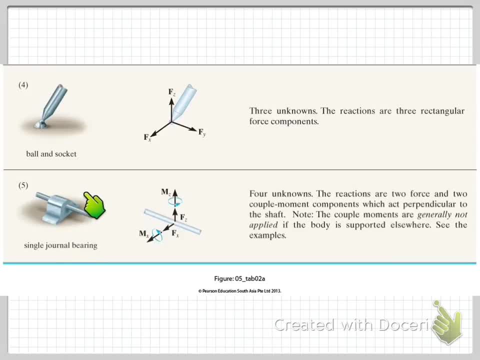 So from this table we can see for our journal bearing here, the shaft is prevented from moving in the horizontal and vertical directions, so therefore we have our force reactions. There's no thrust reaction, so it's free to move in that longitudinal direction. so on the coordinates we've got here, there's no Fy. 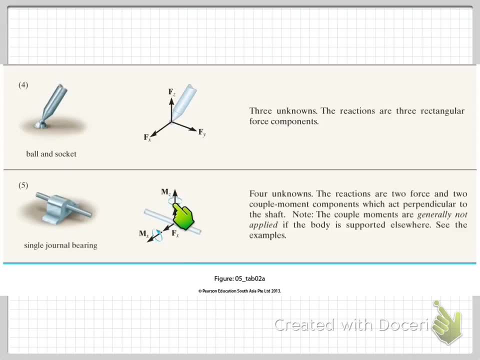 There's no force that goes up or down according to and C type of reaction force, And also you can see here that it's showing that there is some restraint against turning. So we've got a moment reaction. but take note of what it says in here. 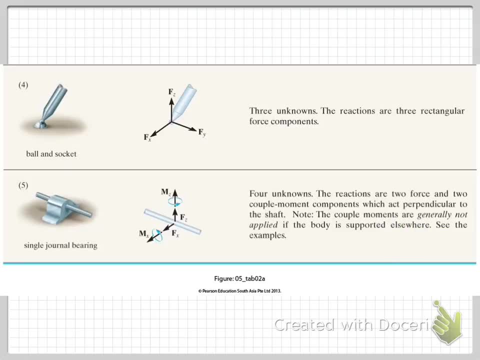 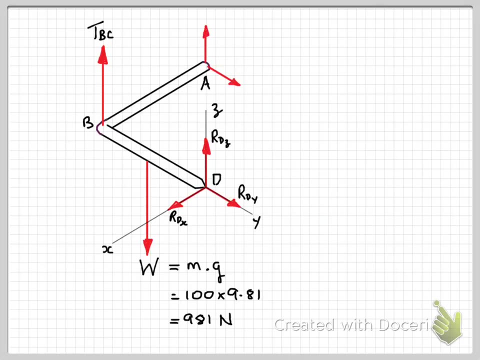 If the body is supported elsewhere, then we generally don't apply the moments as reactions. Okay, so on our free-body diagram, Then We can start drawing in those forces. So So for our journal bearing, it's constrained from moving laterally in the Y direction and in the Z direction. 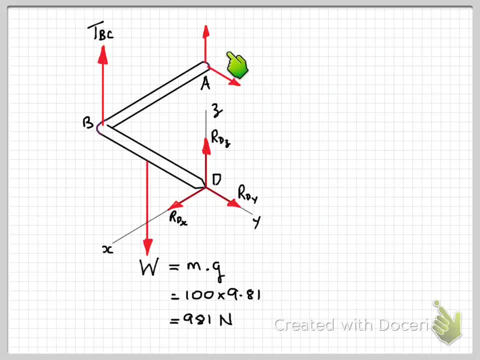 but it's free to move in the X direction. so we have no force there And, as we just discussed, we're not including any moment reaction. Again, we've just assumed a direction for the sense of the forces and then we can put on our labels for those unknown reaction forces. 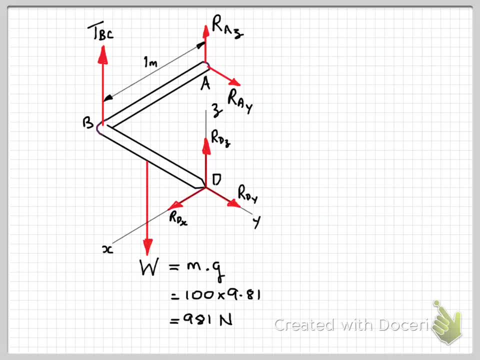 Because this is a rigid body mechanics problem and we're going to be dealing with moments, we'll need some distances, so let's put those on our free body diagram for reference. So in this problem we have on our free body diagram we have six unknowns. 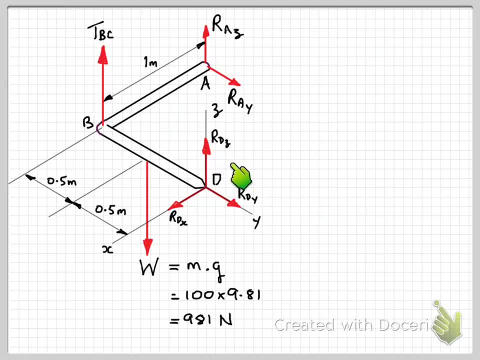 So one, two, three, four, five, six In rigid body equilibrium problems. generally we will start by using a moment equation, So look for somewhere to take moments about, so that many of our unknowns have a zero moment effect about that particular axis. 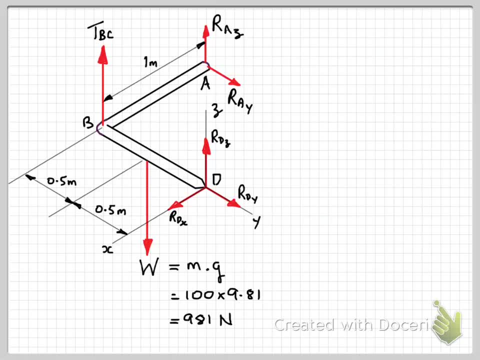 so that they drop out of the equation. So in this particular problem, if we take the Y axis, okay, all of these forces are going to be in the Z direction. So our unknown TBC, our weight force, the reaction forces at D, all pass through the Y axis. 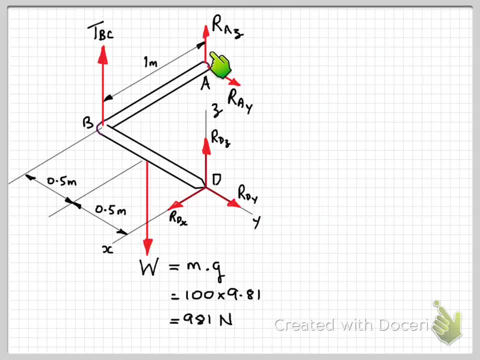 so they have zero moment and we can then leave RAZ as our unknown. So, as I said, there's many different ways to solve these problems and I'm going to go through a fairly simplistic approach which doesn't require too much insight. 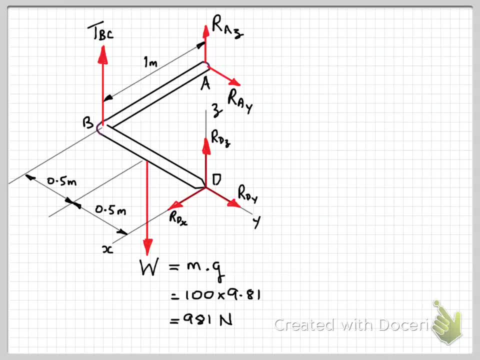 If you're clever and have done a fair bit of mechanics before and you're reasonably good at it, what you might realize is that if we take moments about an axis that passes through the points A to D, take a moment about that axis, then we have our unknown TBC. 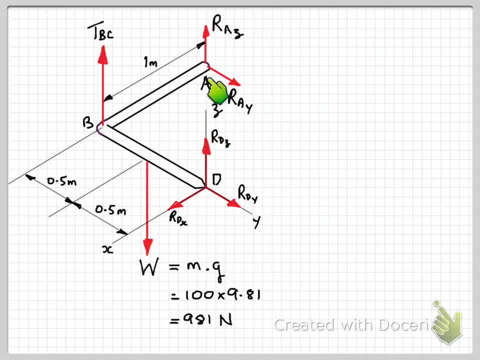 so we just need to work out the perpendicular distance from B to the axis from A to D. and then we have our Y axis weight force and we just need to work out its perpendicular distance from the axis a to d, and that would enable us to enable us to find t b, c straight away. but let's continue on with. 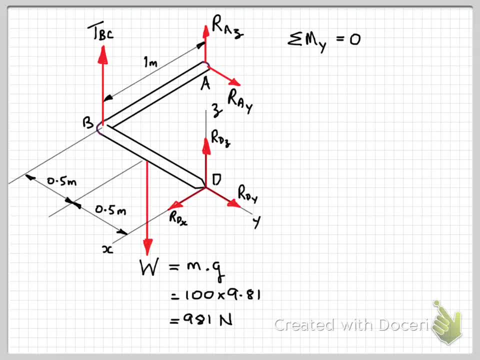 my simplistic approach and we'll take some of the moments about the y-axis as our starting point. so we've written my equilibrium equation. so generally we need to indicate which direction we're taking as positive, clockwise or anti-clockwise. in a 3d problem that becomes a 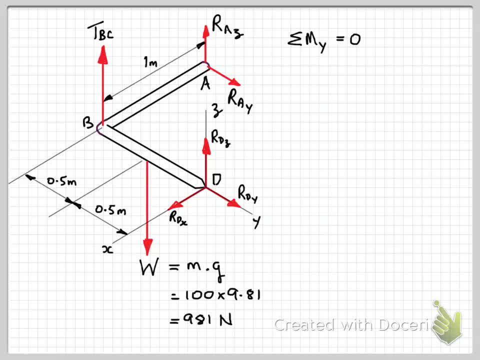 little bit tricky depends on which way you're looking down the axis. so i'm going to say anti-clockwise is positive or counterclockwise positive if you look down that axis at the positive directions of the other two coordinates. okay, so if we have an anti-clockwise rotation, 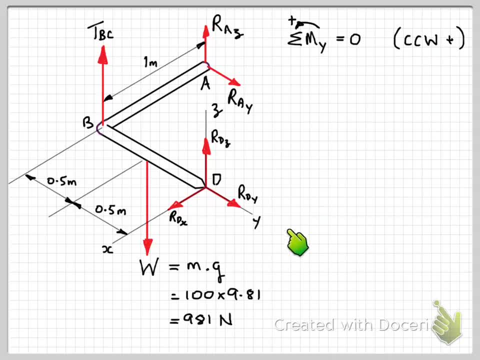 around the y-axis here, looking down that y-axis from the positive side. that's our positive moment. all right. so if we start looking at the forces that have a moment about the y-axis, as we discussed, all of these forces here all act through the y-axis, so they will have a zero moment. 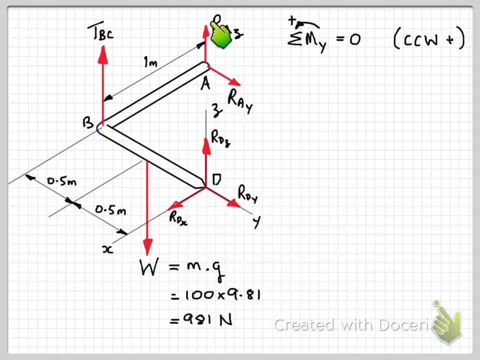 so we've got these two forces out here. now r a z acts perpendicularly at a distance from this y-axis, so that will have a moment effect. so we can write that in r a z times its perpendicular distance is one. and if we consider this force, 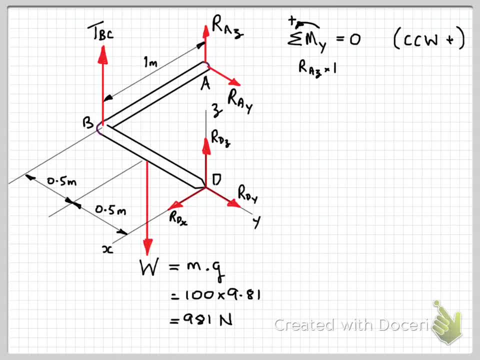 here r a y. even though it's acting away from that y-axis, it's actually. its line of action is parallel to the y-axis, so therefore it will also have zero moment. so we can write our complete equation here: r a z times one equals zero. so of course r a z is equal to zero. all right, so let's use another. 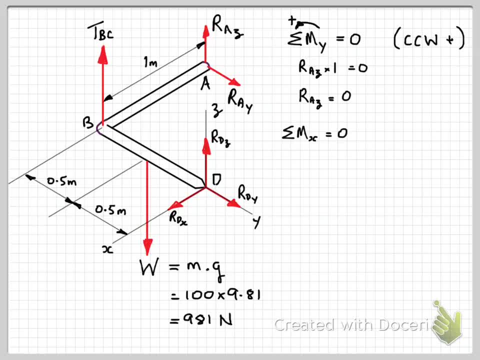 moment equation and we take moments about the x-axis now. so that will give us our known weight force acting in that equation, plus our unknown tension in the cable and also our reaction force r a z, which we've already worked out to be zero. so again, we'll take counterclockwise. 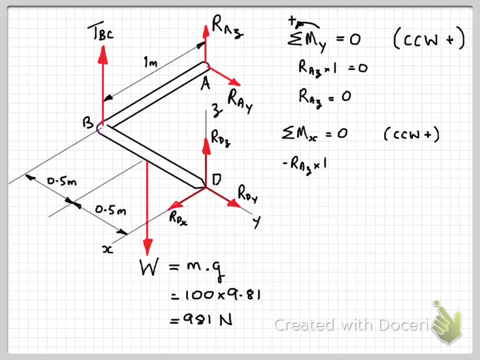 as positive. so we'll have r a z. its perpendicular distance is one and it's going clockwise about the x-axis, so that's negative. yes, we know it's equal to r a z is equal to zero, but we'll just leave it in there for now. we have our force t b, c acting perpendicularly to the y-axis at a. 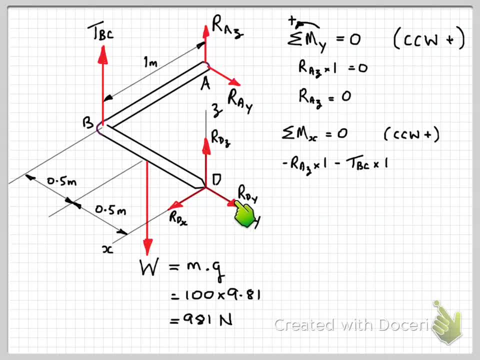 distance of one. again that's going to rotate this thing clockwise about the x-axis. so that's a negative moment and we have the weight force acting down here at a distance of point five and that's going anti-clockwise about the x-axis and all that's equal to zero. so we can solve for our 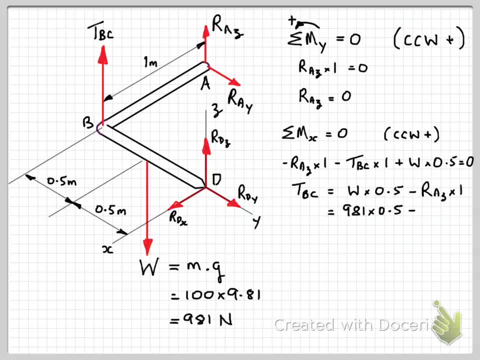 unknown force, t b, c in the cable and we get 981 times 0.5 for our weight force acting down. here we've substituted r a z equal to zero, so we get the tension in the cable is 490.5 newtons. okay, so now we can start working out some of our other reaction forces. so now, if we take moments, 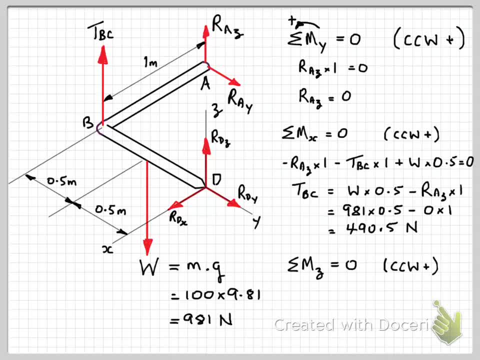 about the z-axis here. the only force that will be causing a moment about the z-axis will be r a y. okay, all of these forces pass through the z-axis. w, t, b, c and r a z are all parallel, so the only thing we need to worry about is r a y times one. 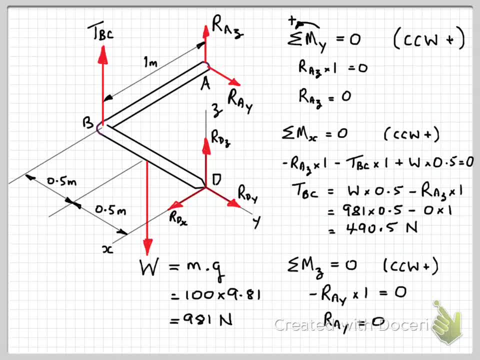 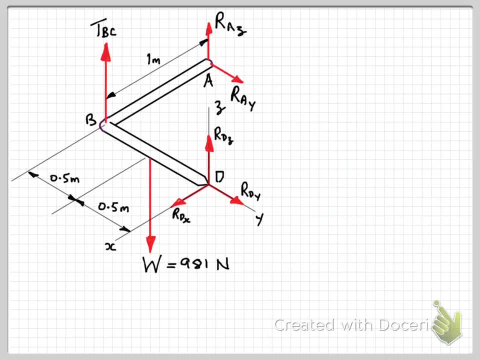 and of course, that gives us r a y equals zero. okay, so let's continue on to find our other unknown reaction forces and we just repeat over here on on this page for references, the things that we've already calculated. okay, so we've used three moment equations, so 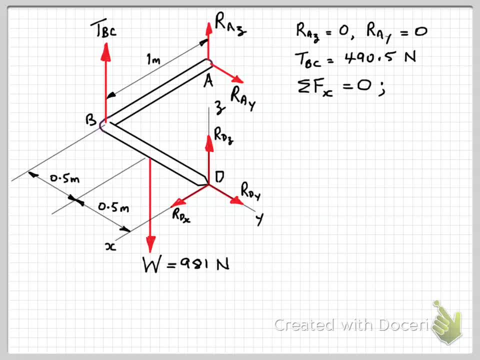 now we need to start using the force equilibrium equations. so let's start with some of the forces in the x direction. and, of course, the only force that we've got acting in the x direction is r d x, so we can immediately write: r d x equals zero. 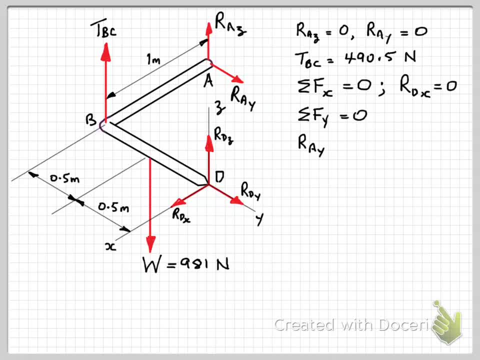 okay, next we'll do some of the forces in the y direction equals zero, and we have r a y plus r d y equals zero. okay, so that's actually Paper for At the danger. So RAY here and RDY are our only forces acting in the y-direction. 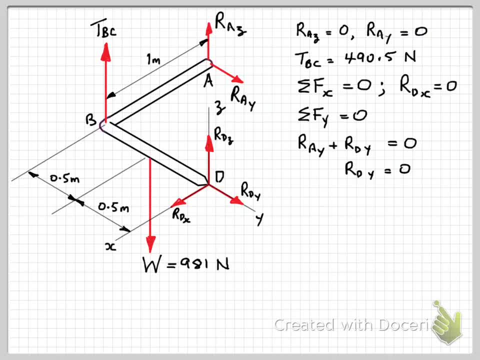 And we already found RAY equals 0 on the previous page, So that immediately gives us RDY equals 0.. Okay, so now let's use some of the forces in the z-direction: equals 0. And we have RAZ our force up here. 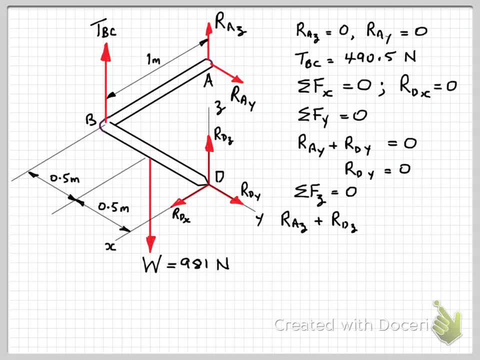 And we have RDZ plus our cable tension and our weight, all equal to 0.. So the only unknown here is RDZ. So let's rearrange that equation and solve for that And we get. RDZ is also equal to 490.5 newtons. 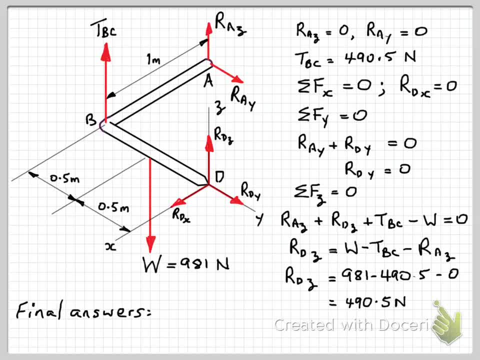 So we've now found all of that And we have our reactions and unknown forces, So we can just write in our final answers. So we had RAY equals, RAZ equals, not RB. Let me just fix that up. Okay, so RAY, RAZ, RDX and RDY, all equal to 0.. 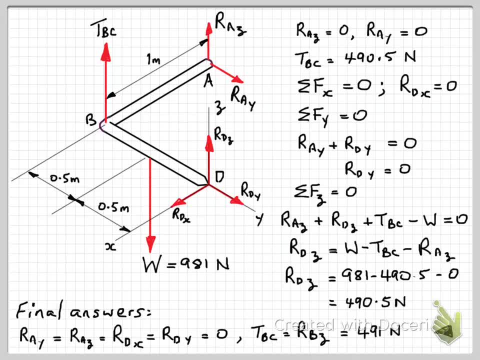 And our cable tension and the reaction force again not B, that should be D, So let me again fix that. Sorry about that. Okay, so tension in the cable and the reaction force at D in the z-direction is 491 newtons. 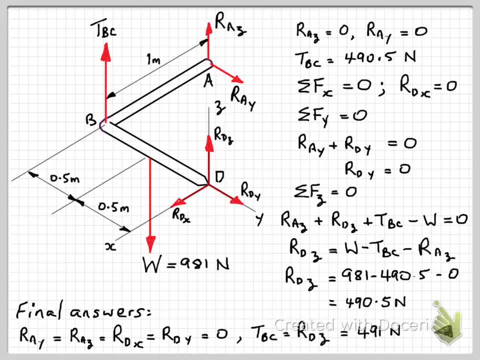 So that's the end of the problem. I hope it's been helpful to you, And please look at some of my other engineering mechanics videos if you need more assistance with solving engineering mechanics problems. And, just as I said at the start, this is not the most elegant way to solve this problem.